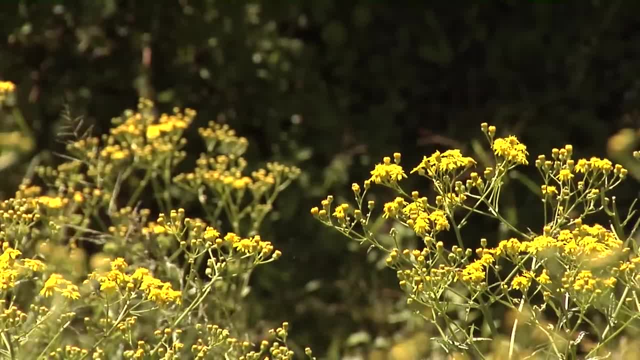 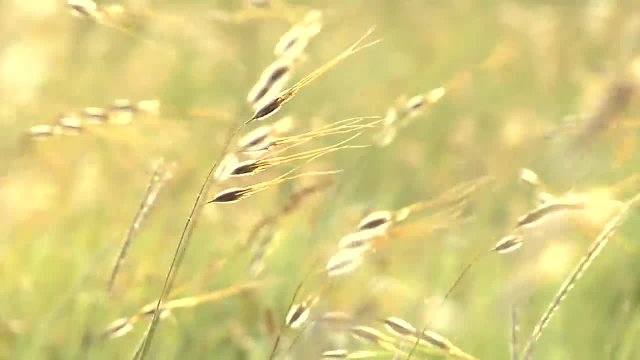 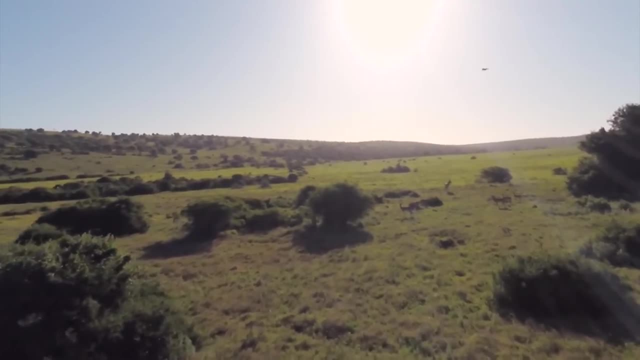 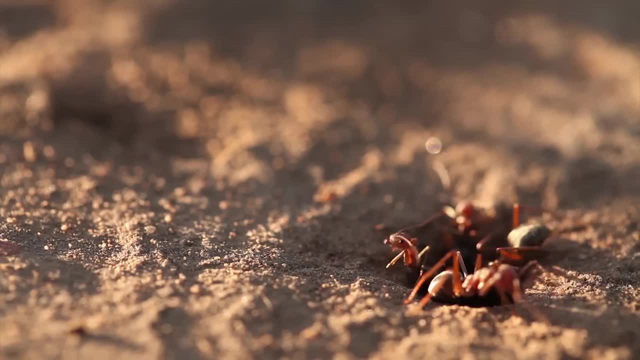 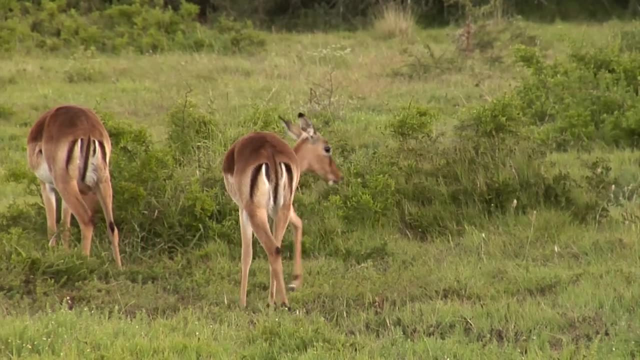 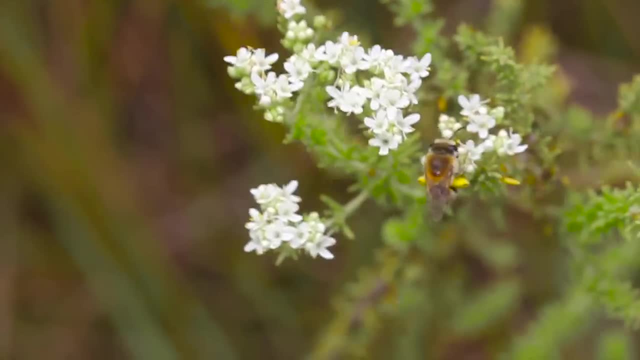 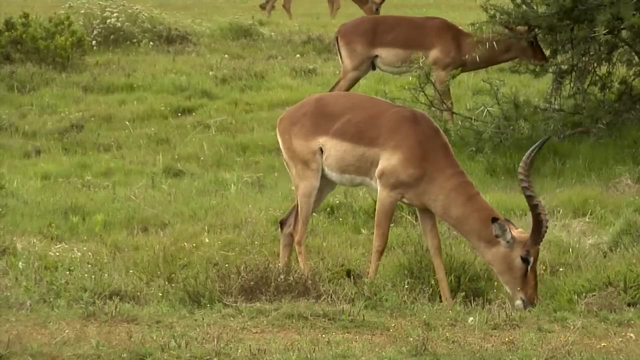 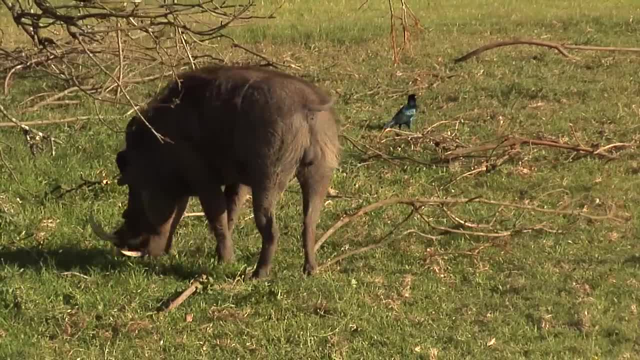 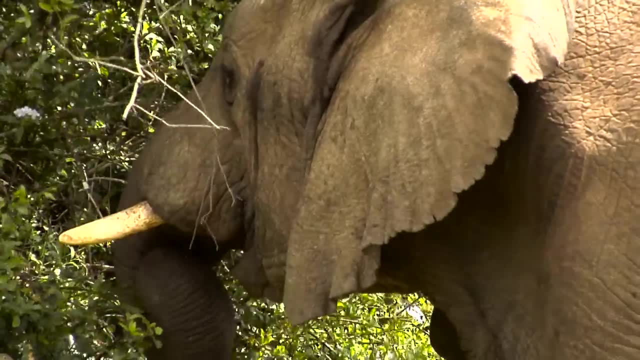 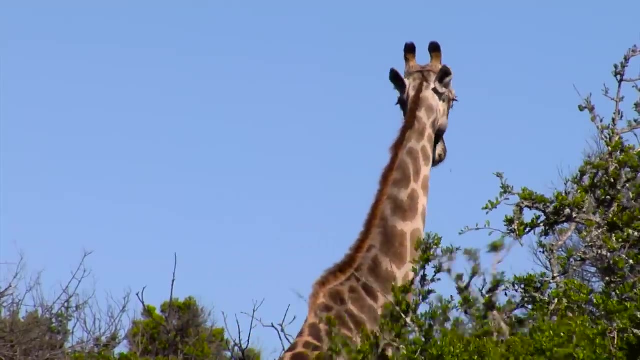 Water muffles dig for roots and grubs in the shallow dirt, Elephants browse on trees and bushes, And the giraffe, towering above all, grasps leaves from the tallest trees, each species playing an essential role in maintaining the African savannah. 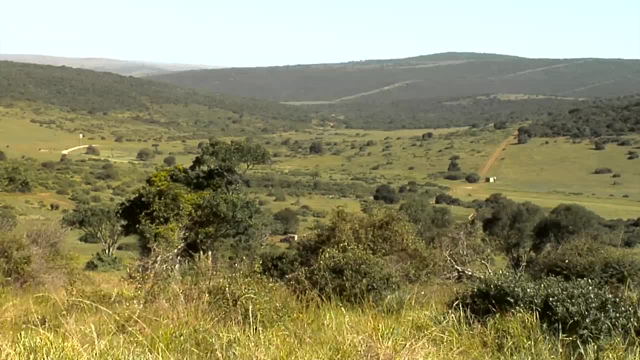 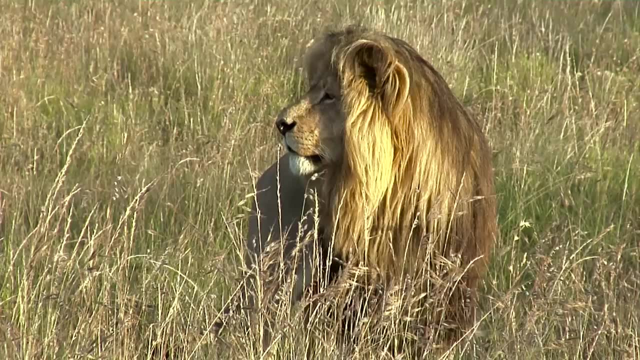 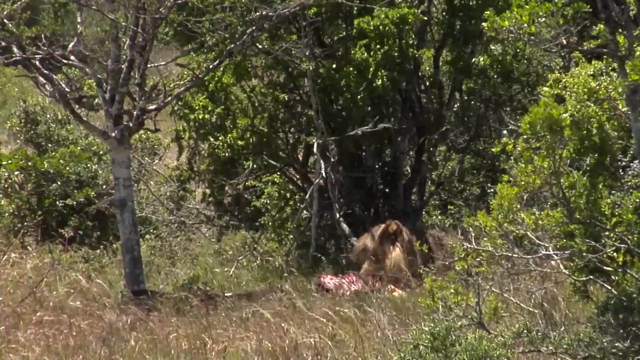 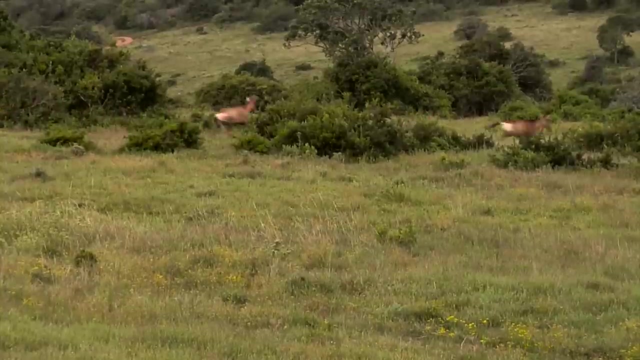 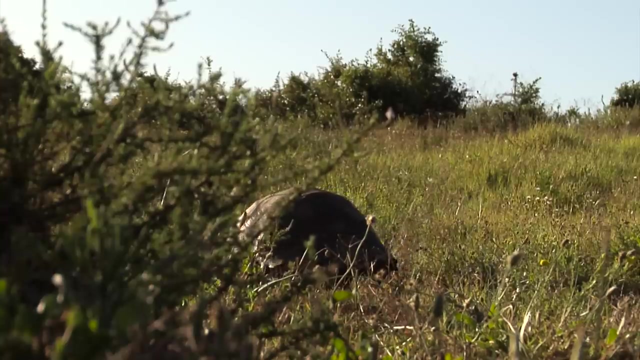 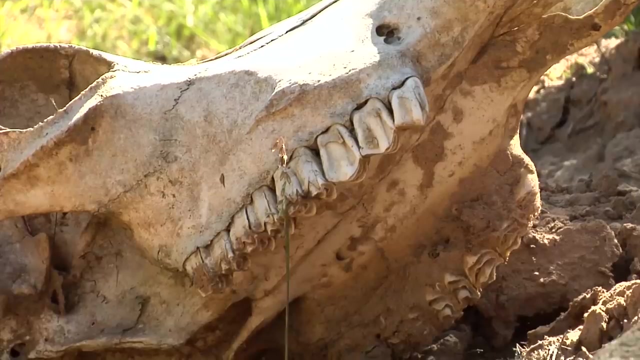 Watching are Africa's predators, the king of which is the lion. Their role is to regulate prey, removing the weak. Thinning out large herds of animals opens up space and resources for smaller herbivores. Death is an inevitable part of the cycle, yet energy is not lost. 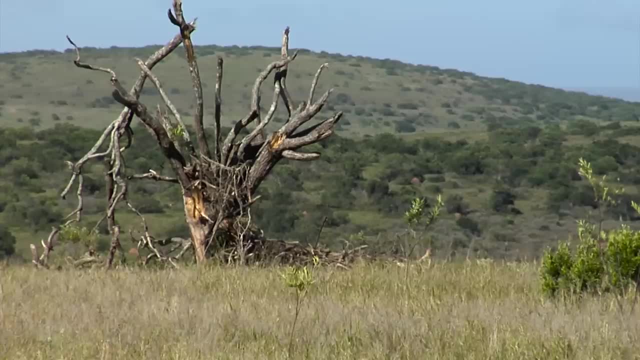 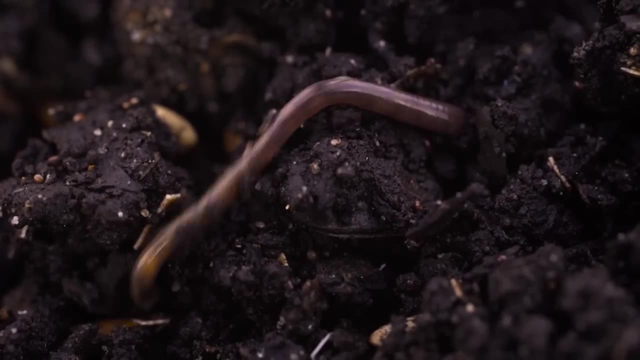 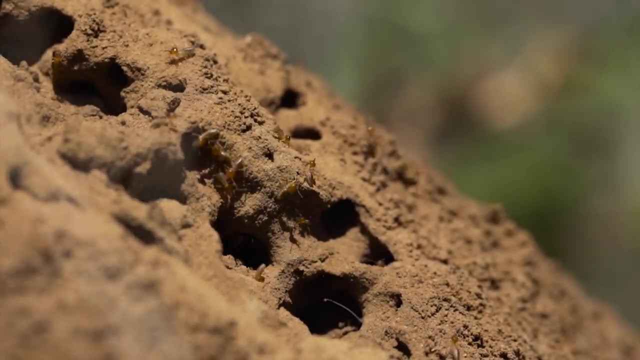 Carcasses release a torrent of vital nutrients back into the delicate ecosystem. Centipedes, worms and bacteria thrive on these rich nutrient deposits. Termites, always busy, are another major decomposer of the savannah, returning nutrients to the soil as they grow. 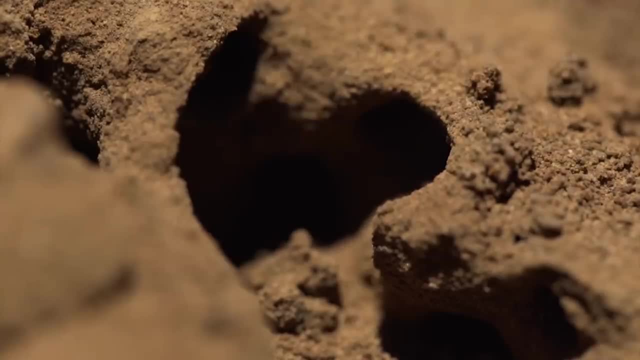 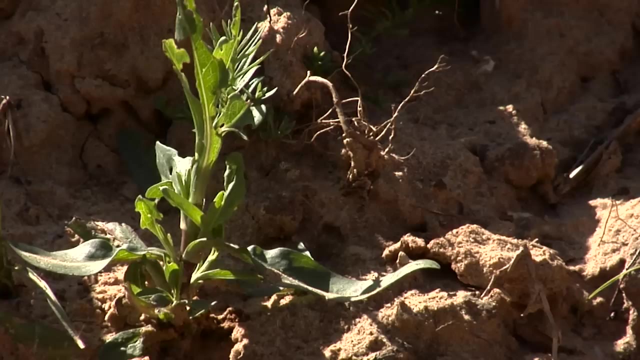 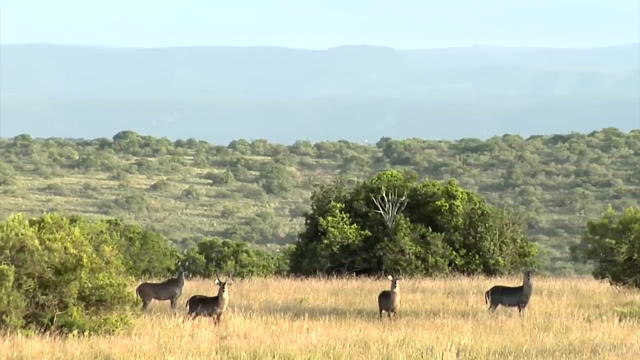 Termites, always busy, are another major decomposer of the savannah, returning nutrients to the soil as they grow And as they consume dead plant matter. These nutrients are now ready to enter back into the cycle. Up through the roots of plants, they are drawn, shoots, sprout, flowers, bud, and the trees grow stronger and taller.